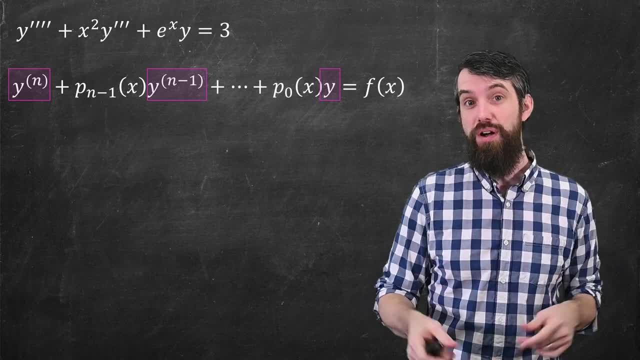 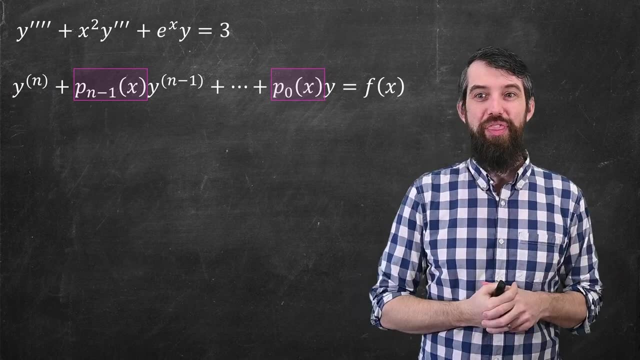 that they're linear And that just means that we're adding the higher order differential equation to the higher order differential equation. up these functions, But with coefficient functions out the front. my standard labeling here is to put a 1 in front of the nth derivative But then in front of the n minus 1th derivative. I call it. 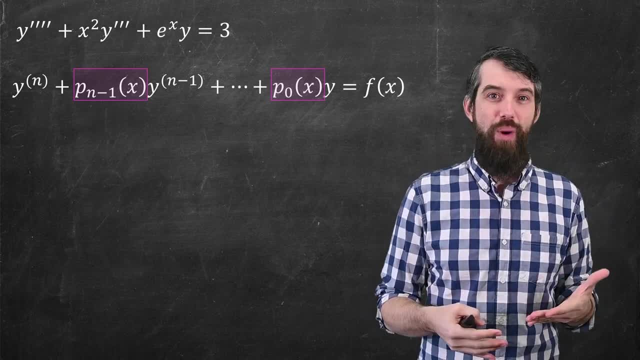 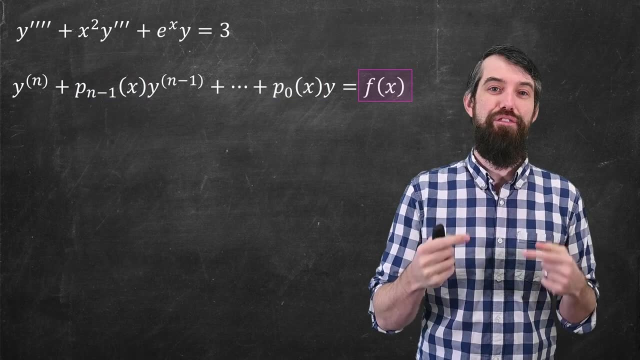 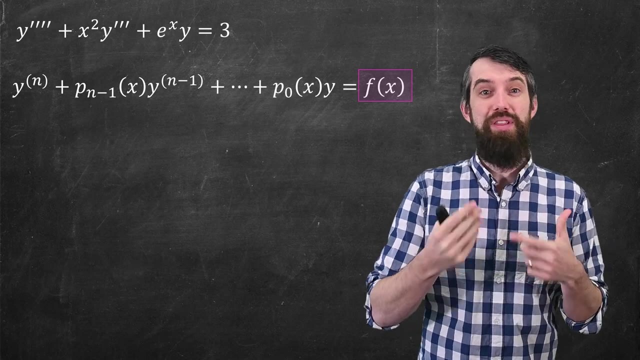 the coefficient function p sub n minus 1.. And all the way down to y, which is sort of like the zeroth derivative, I put the coefficient function p sub 0. And then, on the far right hand side, I have this f of x, And if this f of x was 0, that's going to be important to our theory a. 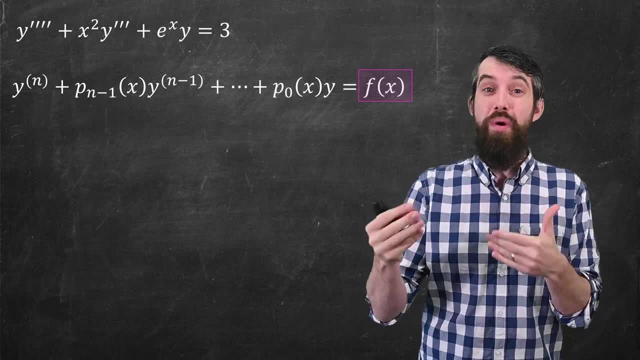 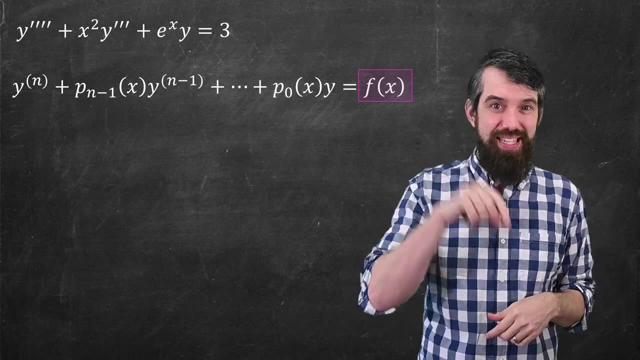 lot of the theory in the nth order case is really going to be going in parallel to the theory that I've already talked about in the second order case. So I'm going to link down in the description the second order theory video. So if you really want to dive into that video first and then come, 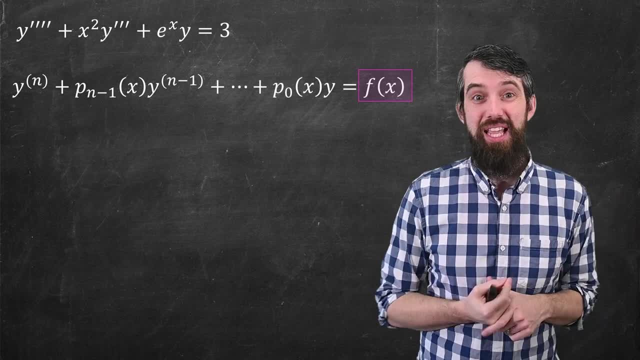 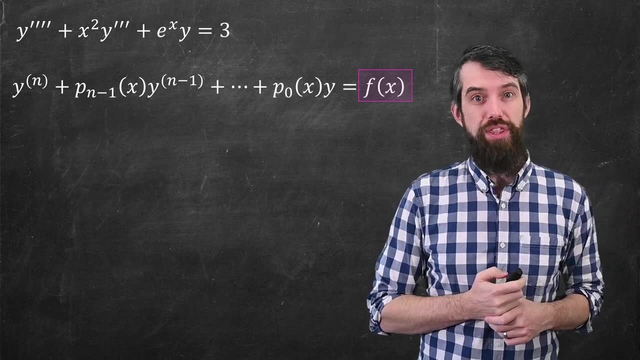 back here. that's not a bad idea, But but a lot of the ideas are actually pretty much the same, So you're welcome just to stick with this video as well, if you prefer, in the nth order case, All right. so let me state my first theorem that's relevant for such differential equation. This is: 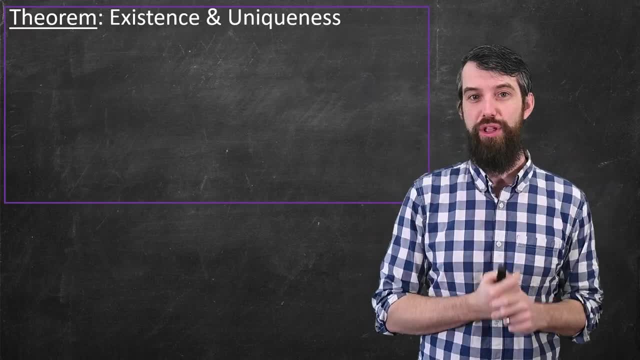 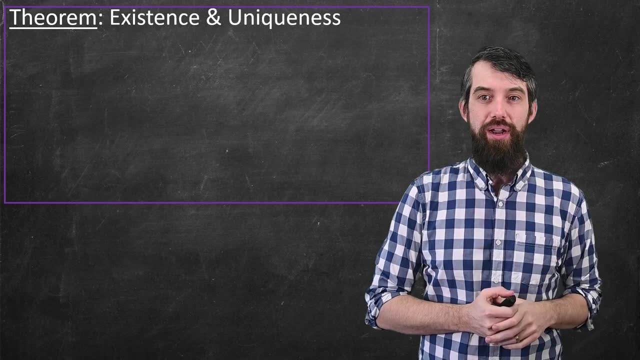 my existence and uniqueness theorem. This is my existence and uniqueness theorem. This is my. the key thing that makes differential equations worth. it says this is when there exists a solution and even better, when that solution is unique. So the context here is: I start with an. 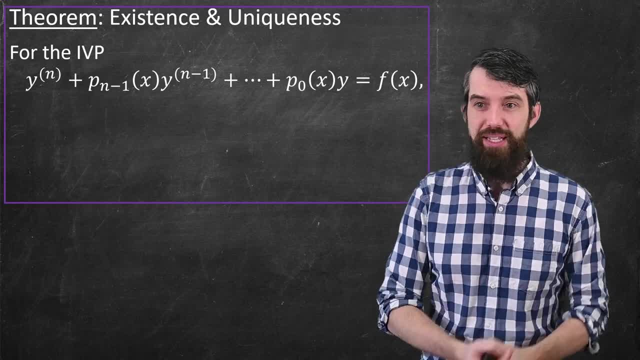 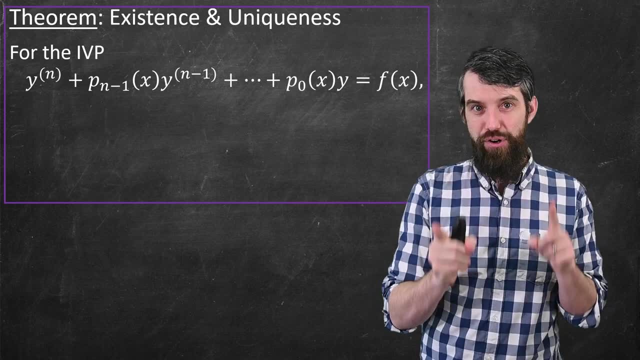 initial value problem. in IVP. An initial value problem consists of a differential equation, So here I'm assuming a linear differential equation together with initial conditions. Now this is the first spot where things change, Because this was an nth order differential equation, highest. 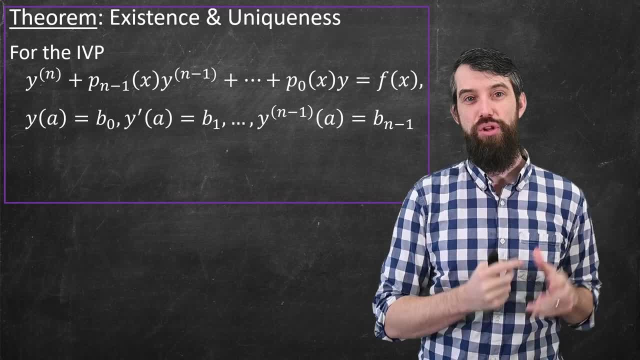 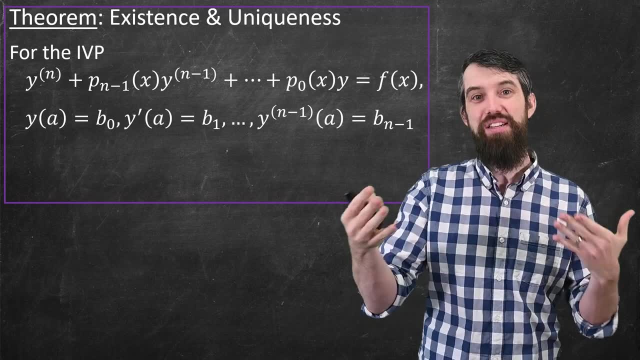 derivative was n, I need to have n initial conditions As well. So you'll notice I have b zero up to b, n minus one, zero up to n minus one, that's n different conditions. So for example, if it's second order, you need two initial conditions. If 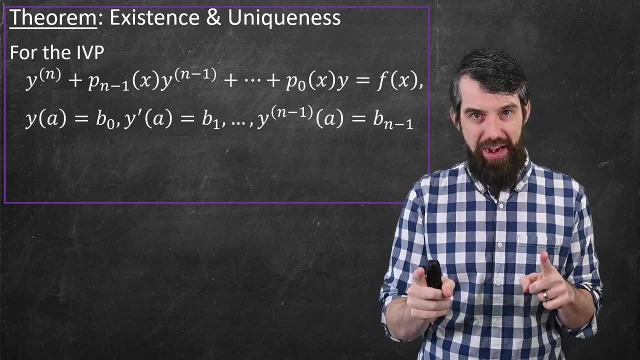 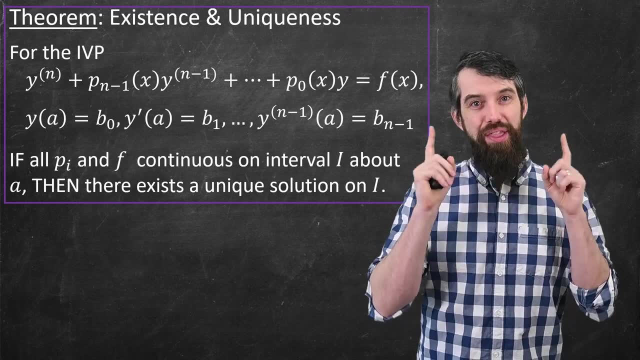 it's 10th order. you need 10 initial conditions. then, provided everything is nice, like the coefficient functions, the pi and the f are continuous on some interval, then the existence and uniqueness theorem guarantees that, yes, there exists a solution And that solution is unique. 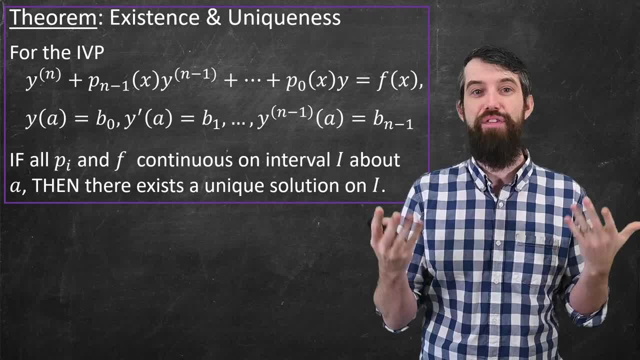 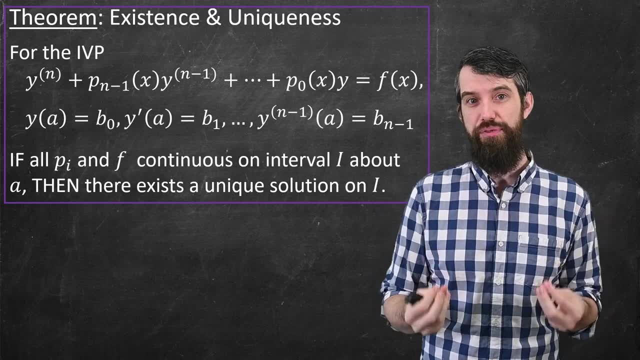 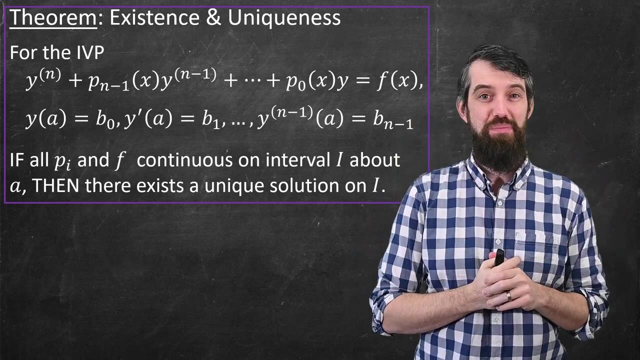 on the entire interval where you're coefficient functions and your f are nice. So we have this pretty strong existence and uniqueness theorem. that's true for higher order linear differential equations like this one And indeed, other than jumping up to n initial conditions and nth order differential equation. this is really 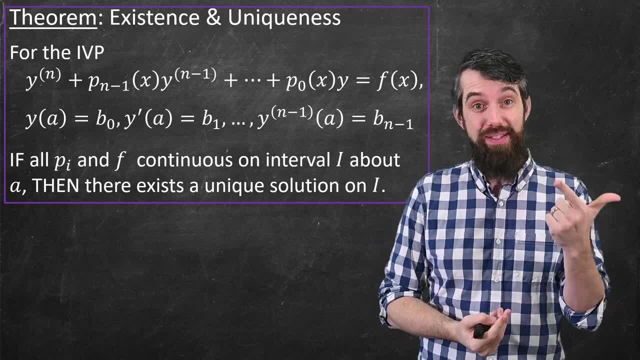 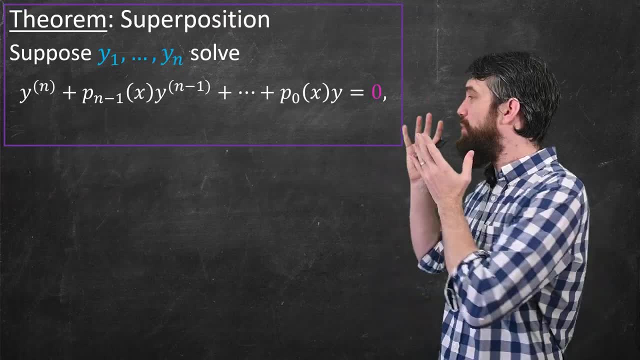 the same thing that we've seen now three times. We saw it in the first order, we saw it in the second order and we saw it now in the nth order. The next point is one that we've also seen back when we're talking about second order. It's the principle of superposition, And this is the idea. 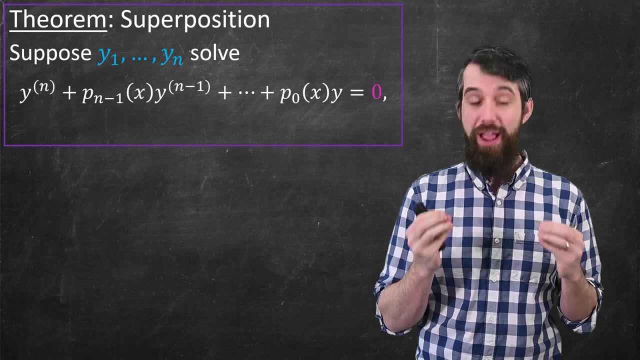 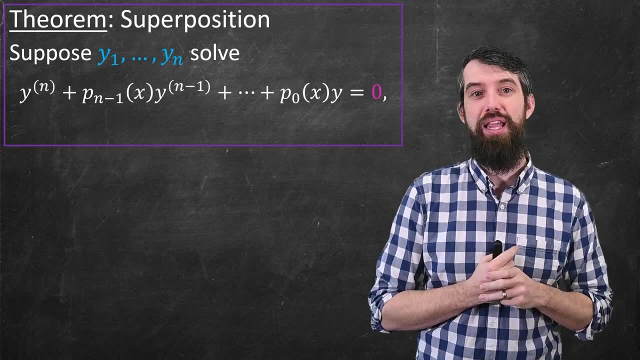 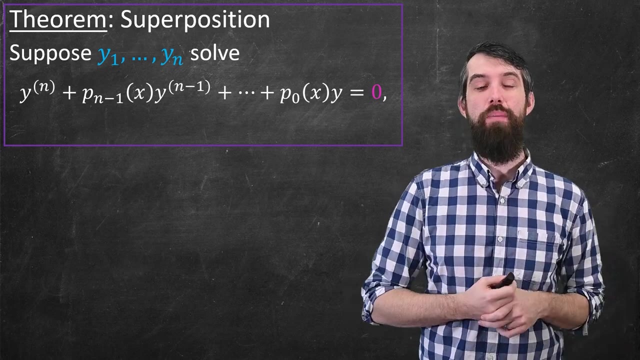 Imagine you have n solutions to an nth order- and this is important- homogeneous differential equation. Homogeneous meaning the right-hand side was equal to zero, as I've highlighted in pink. Then the idea is this: If you found n solutions, you could take any linear combination of those. 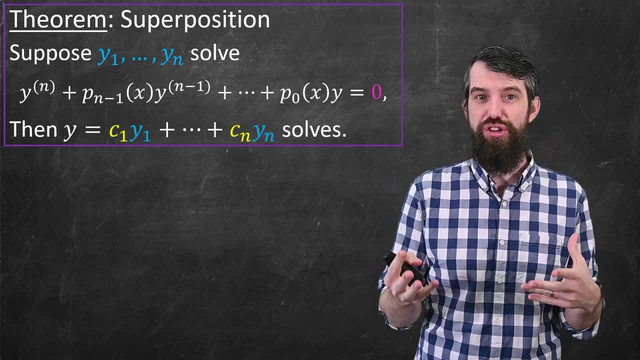 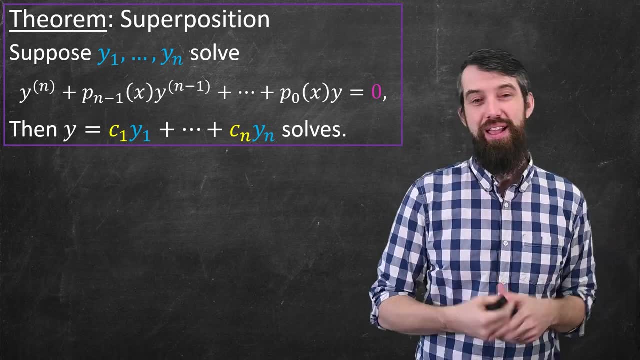 c1, y1 up to cn, yn- any linear combination that you wish and that also solves the differential equation. The basic idea is that since my equation is linear and derivatives are linear operators, then this all just plays really well with taking a linear 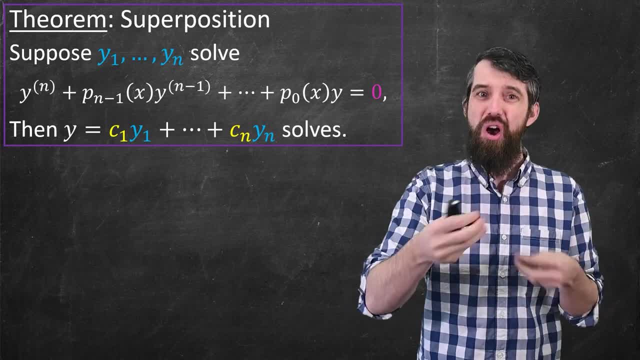 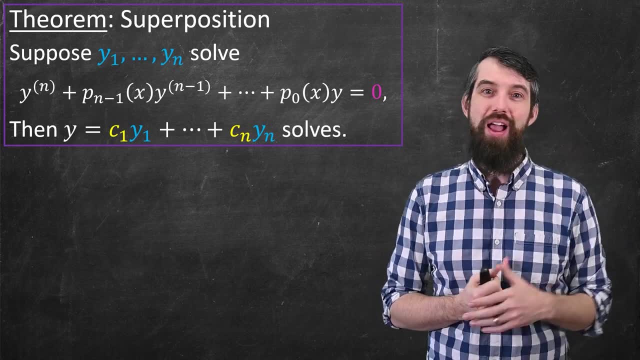 combination. Everything works together, So you find any solutions. linear combinations of them are also solutions. This is extremely powerful, because if you didn't have a theorem like this, you could go and find one solution. you can find two solutions. you can find a hundred solutions. 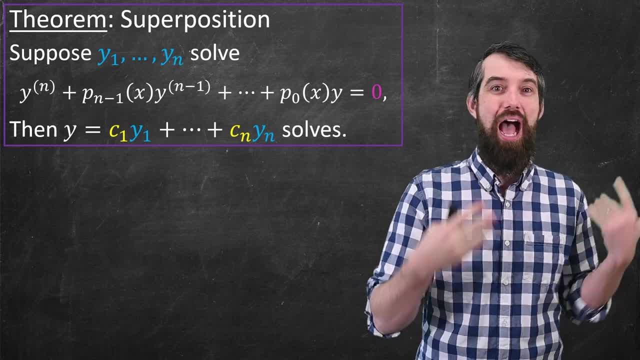 and you'd be like, okay, great, you found a hundred, but there could be infinitely many. How do you find all the others? Well, this is going to get us a long way to being able to rapidly expand all the solutions that we can find. 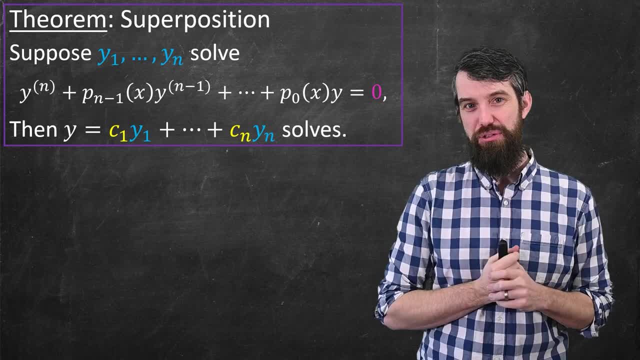 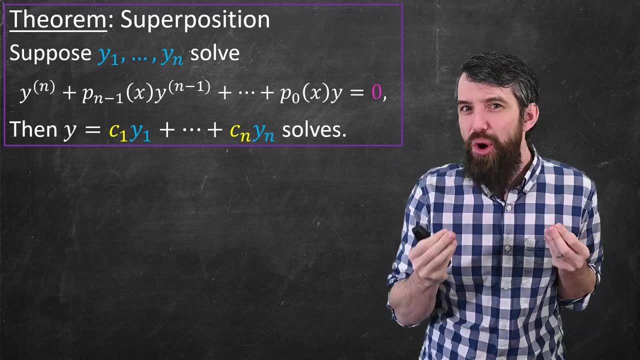 Isn't quite enough, Because if you've gone and found n solutions and then using this principle, really what you get is sort of n infinite families, like the linear combinations of those n. you still don't know that you found the ball. Maybe there's more, By the way, 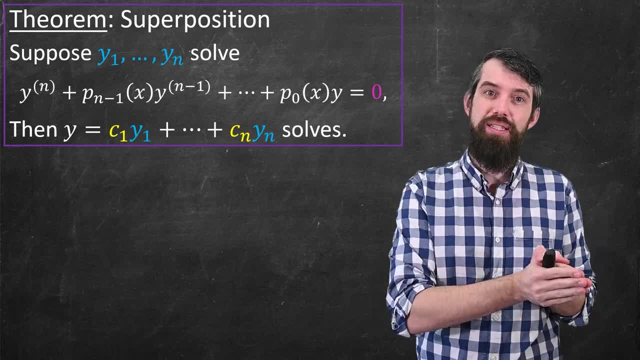 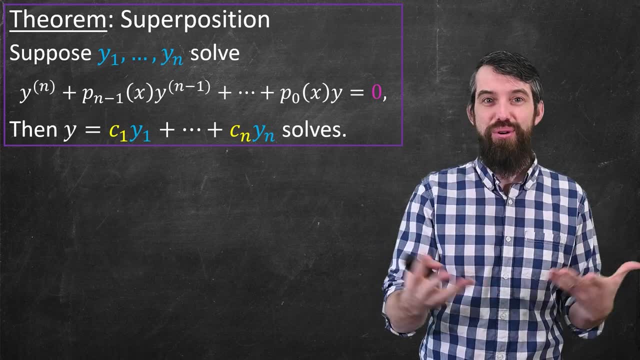 it's good to keep clear the difference between what we're talking about now and existence and uniqueness. For existence and uniqueness, you had initial conditions, so there was only one. Here. I haven't specified initial conditions, so I'm trying to solve the general solution to the. 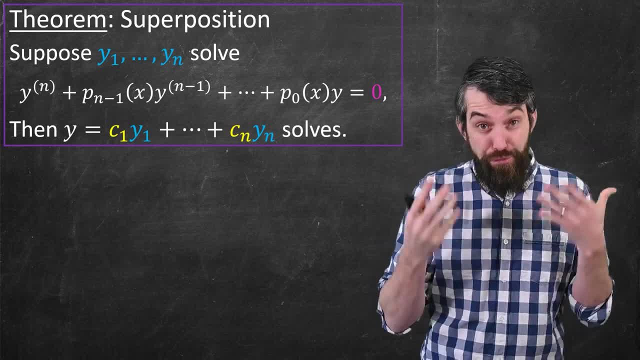 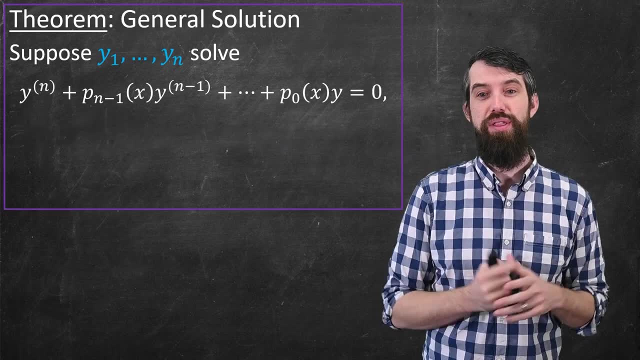 ODE without initial conditions. We could do initial conditions from this at the end. Okay, so now we get to the most important piece, and it's the following. I call it the general solution theorem and it says the following: Suppose you have n solutions to this, 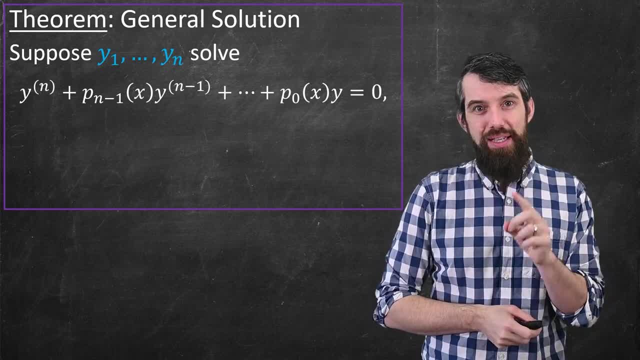 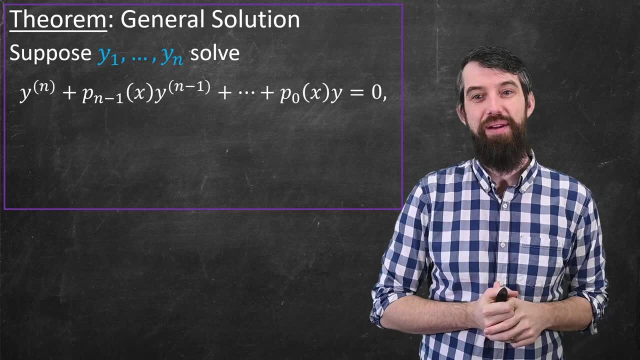 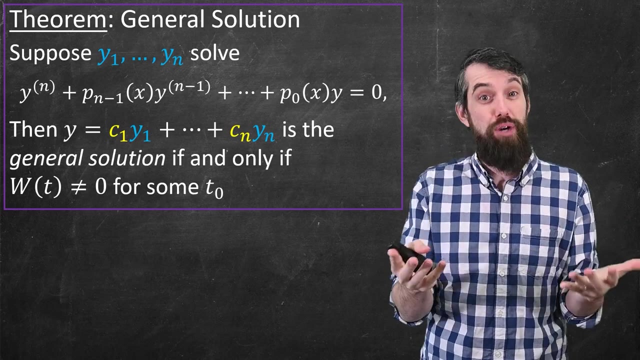 nth order, linear differential equation, Then my claim is that this is enough. This is enough to describe every possible solution, provided some statement about the Wronskian, That is, the linear combination c1y1 down to cnyn is the general solution. General solution means any solution can. 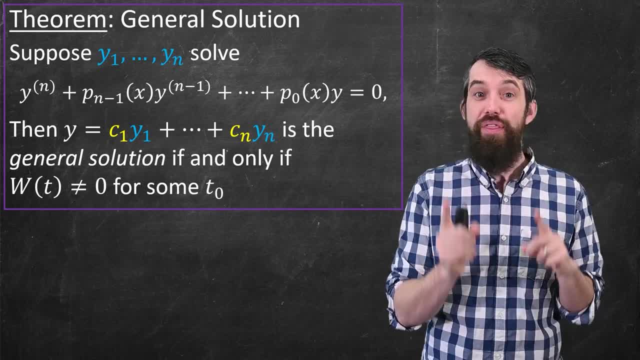 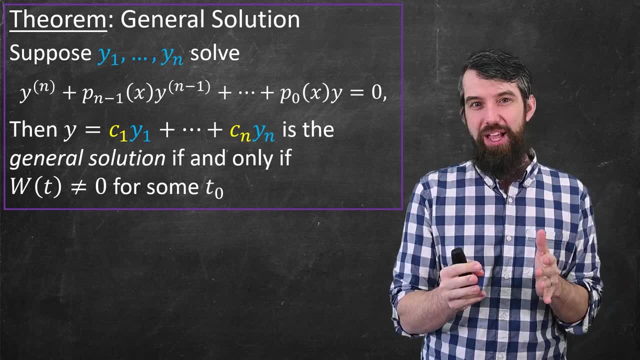 be written in this way. General solution means any solution can be written in this way. General solution means any solution can be written in this way, And that is true if, and only if, the Wronskian of the y1 down to the yn is non-zero at some point, some point t0.. So this is really good, because it now 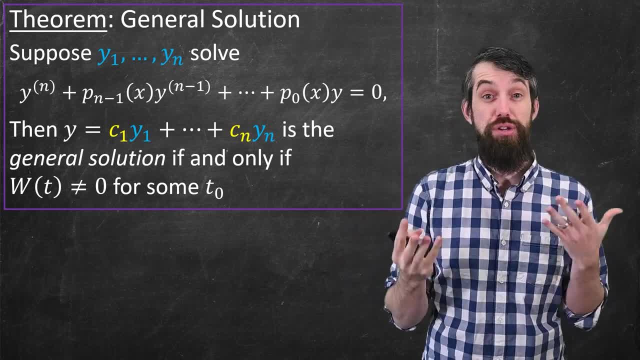 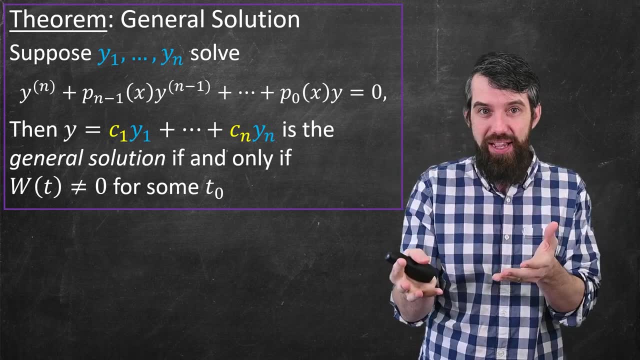 tells you when you can stop searching for new solutions to your differential equation, If you find n of them and you find that those n solutions you've gotten are linearly independent. this is this test we have with this Wronskian. so if you find that you have, 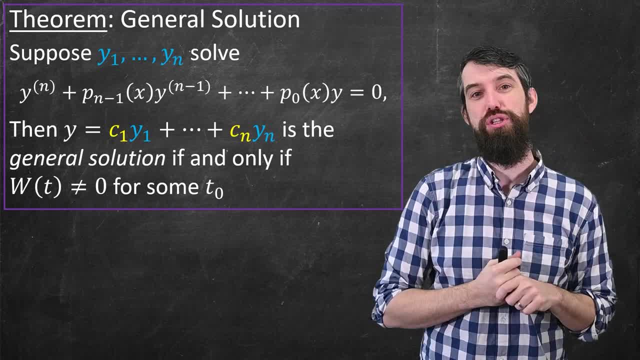 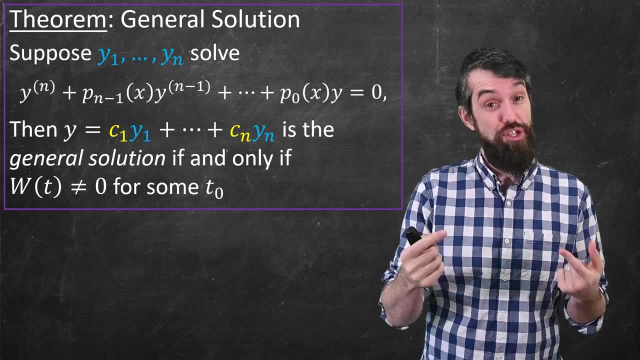 n linearly independent solutions. that's it. Every other solution can be written in this way, And that means you're done. You've solved your differential equation. If you had n initial conditions as well, you could substitute in and figure out the values of the constants. 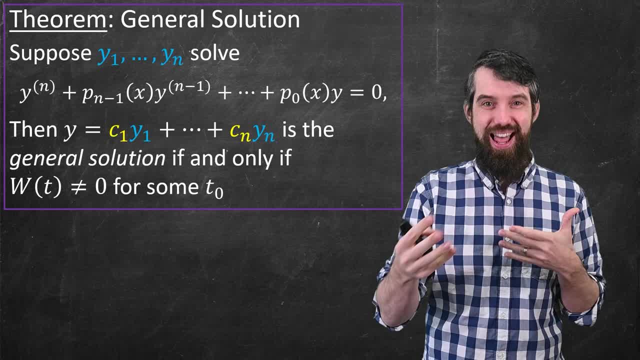 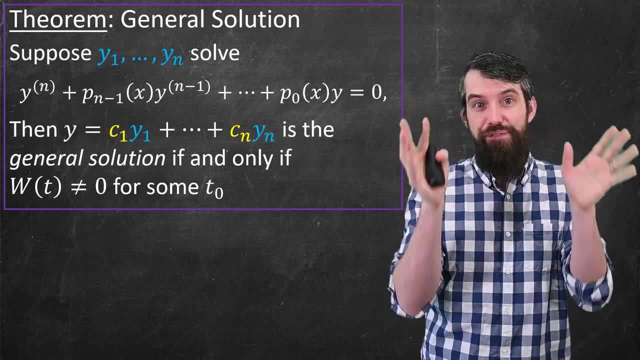 Now for those of you that know a little bit of linear algebra, I want to make the analogy a little bit stronger. We have this wonderful theorem in linear algebra that says: suppose you have n linearly independent vectors. Well, if you live in n dimensions, then the linearly 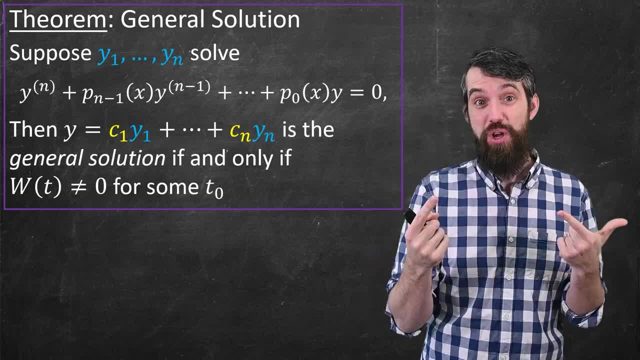 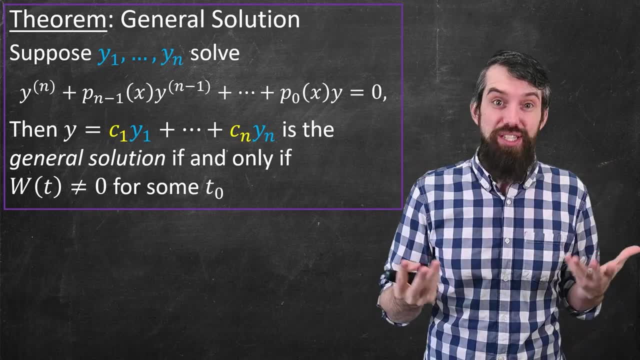 independent vectors form a basis, which means any vector could be written in terms of the Wronskian. So those n linearly independent vectors. Well, it's sort of really the same type of statement. We're imagining that we're living in n dimensions because we've got an nth order differential. 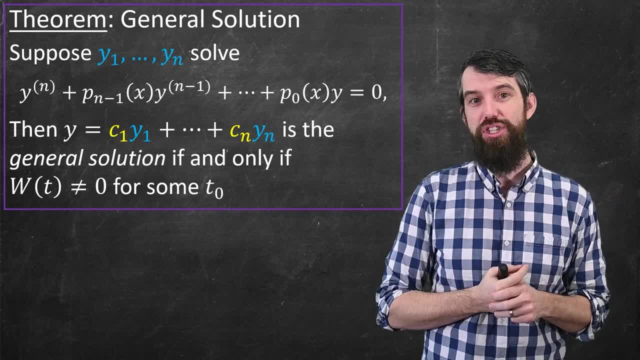 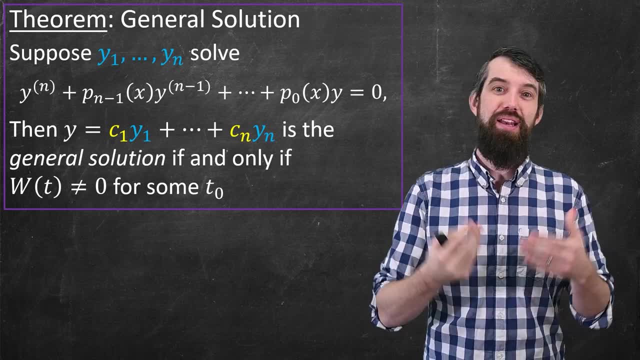 equation And if you have n linearly independent solutions, then the linear algebra word would be to call them a basis, because anything could be written as a linear combination of them In differential equations. we typically call these not a basis, we call them a fundamental set. So 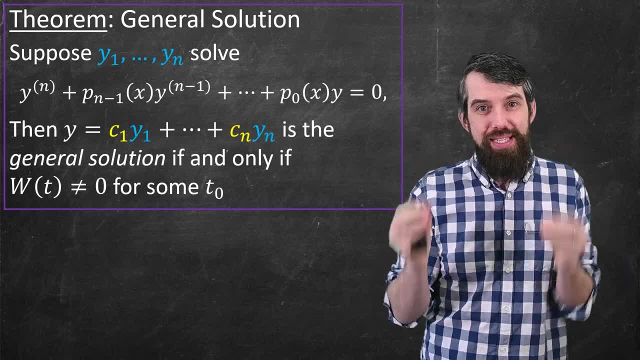 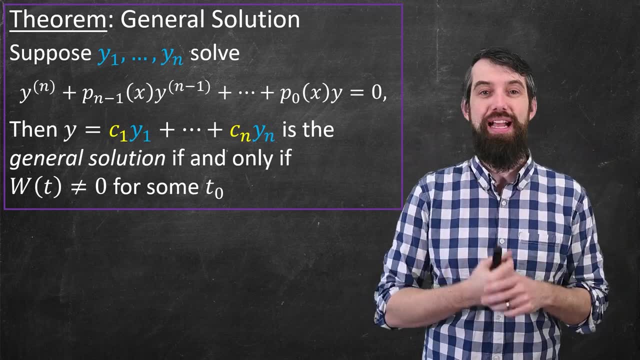 y1 down to yn is called a fundamental set, And this means well precisely what we've written down here: that they're linearly independent and that any solution can be written as a linear combination of them. So this gives us the following method. If I'm 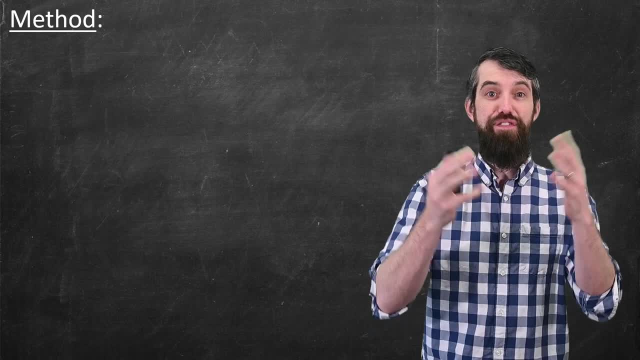 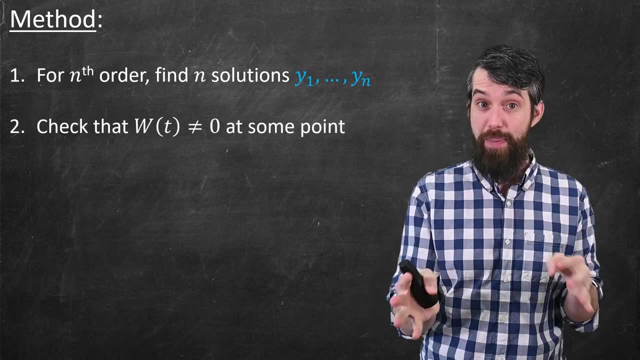 trying to solve an nth order differential equation. what I do is first I need to find n solutions to that nth order differential equation. Then I need to check that indeed those n solutions are linearly independent, which we have a test for. You take the Wronskian.